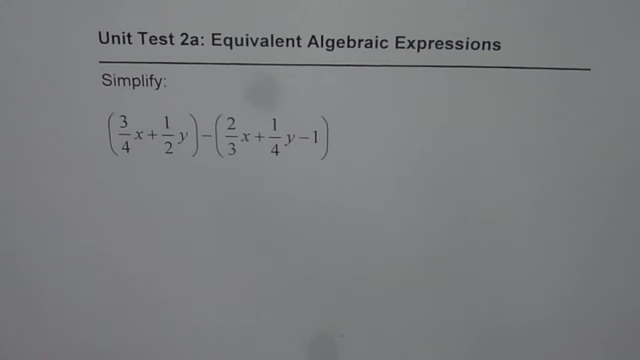 I'm Manil Kumar and we have some good questions here to practice for unit test on algebraic expressions. So in part A of the test we are dealing with polynomial expressions. Here we have an example to simplify which involves fractions, So kind of review for fractions with different denominators. 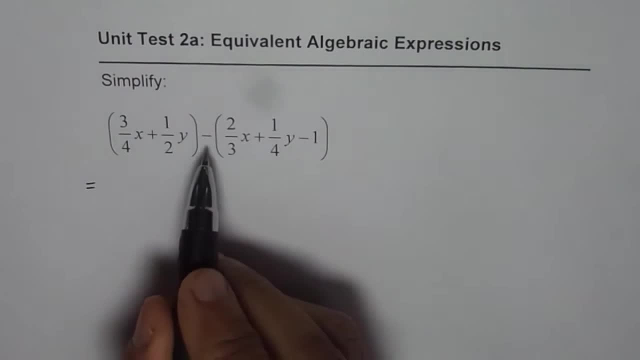 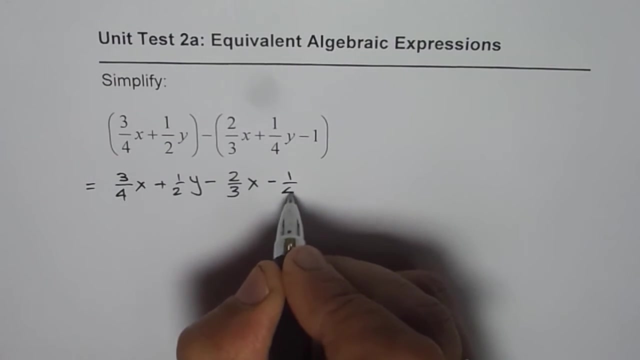 So let us expand this. Rather, I should say, open these brackets and bring the like terms together. So what we have here is 3 over 4x plus half of y minus. all signs will change: 2 over 3x minus, 1 over 4y plus 1.. 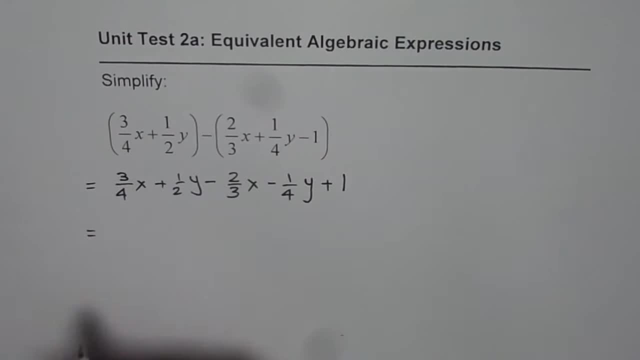 Now let's bring the like terms together. So we have 3 over 4x minus 2 over 3x, plus 1 over 4y. So what we have here is 3 over 4x minus half y, minus one fourth of y plus 1.. Now to add or subtract fractions with different denominators. we should take common denominator Now. for these, the common denominator is 12, right. So we can multiply both numerator and denominator by 3 for the first one, So we get 9 over 12x, and for the second, one by 4.. So we get 8 over 12x. 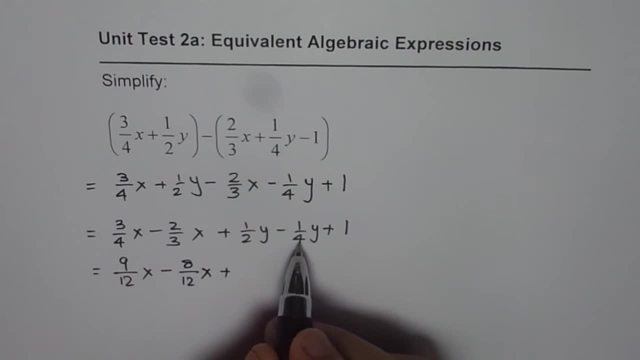 As well as the denominator and denominator. So we get 9 over 12x and for the second, one by 4.. So we get 8 over 12x. As the y is a concern, we need 4 in the denominator. That's the common multiple right, The least common. So we can multiply and divide the first term by 2.. We get 2 over 4y, minus one fourth of y plus 1, right.